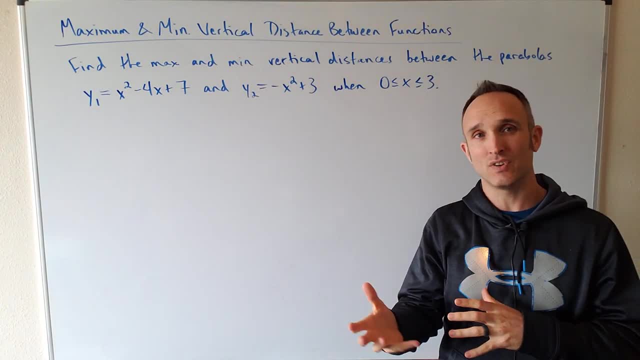 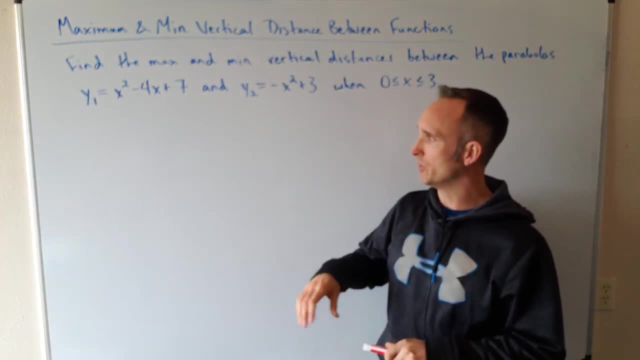 And then we're going to look to minimize that distance between the two functions, And then we're going to look to minimize that distance between the two functions. these are parabolas, so you should be pretty familiar with them. This parabola, because the 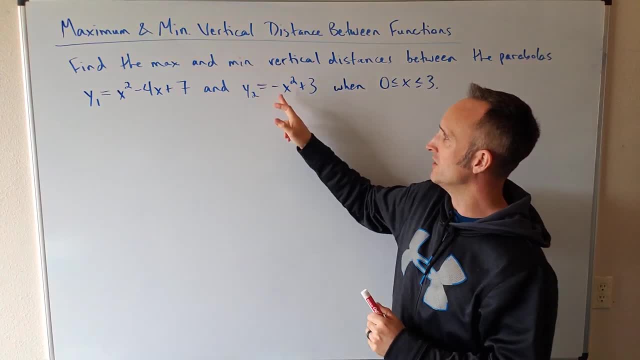 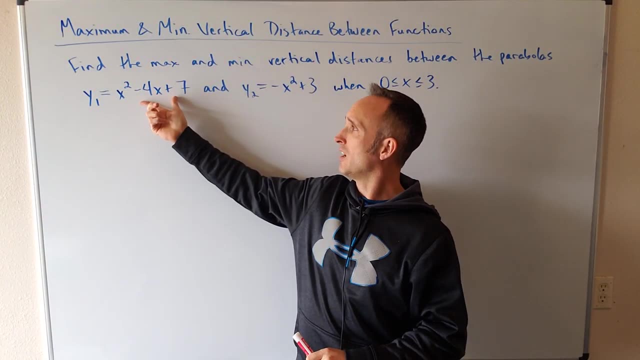 coefficient of x squared is positive, is going to open up, And this parabola- because the coefficient of x squared is negative- means it opens down. In other words, this function is going to be opening up and the other, the second one's going to be opening down. So we could think of this as being: 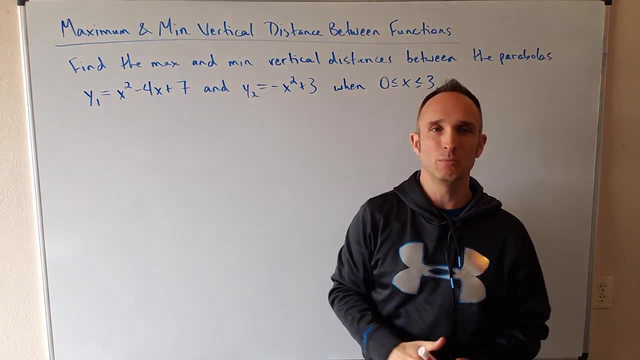 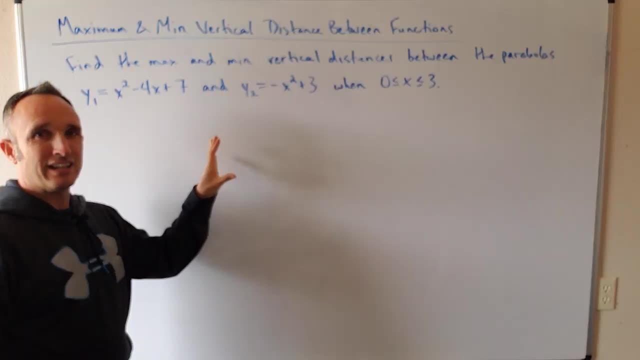 the higher function. So when we calculate vertical distance, that's going to be important to keep in mind. All right, so in this particular optimization problem, we don't need to define any variables, because we've already got all the variables we need. Furthermore, we don't need to define the 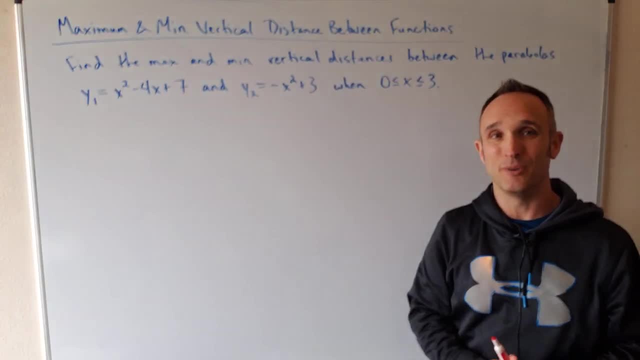 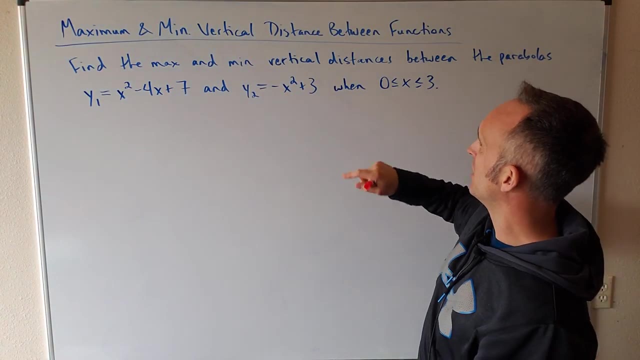 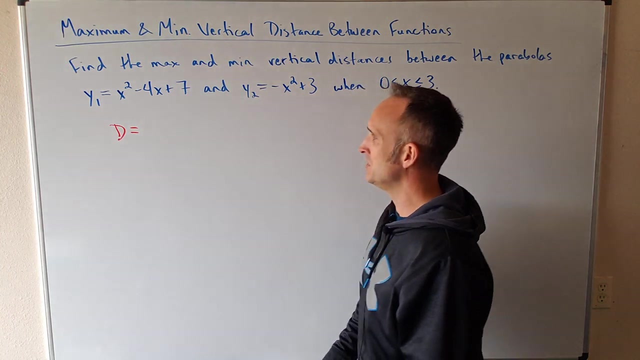 relationships between x and y, because those are given to us as well. So we can jump right to the function that we want to maximize and minimize, And so that's our vertical distance function, which I will call d. So d is the vertical distance between the two functions, If you want to calculate. 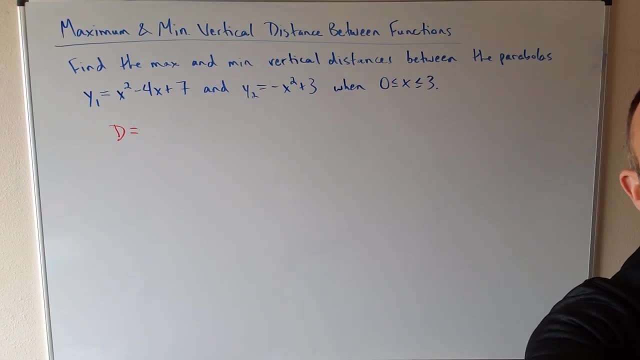 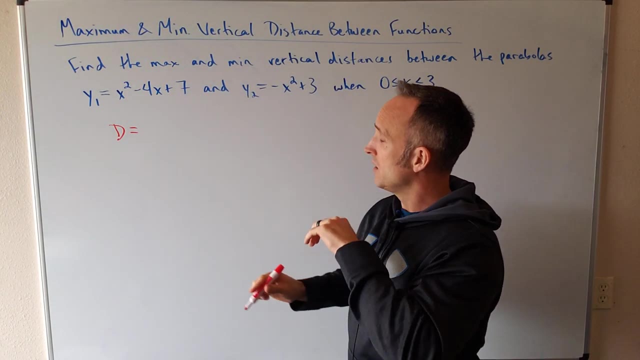 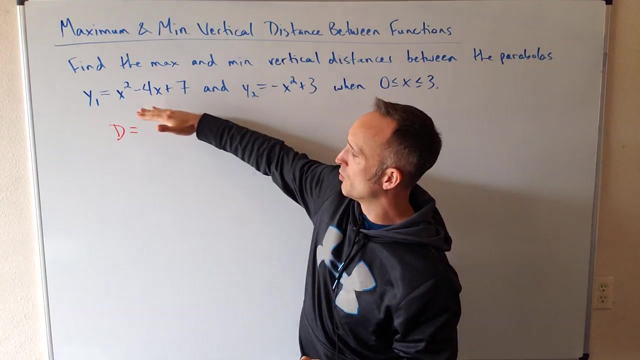 vertical distance. let me turn my auto zoom off. Okay, if you want to calculate the vertical distance between two functions, you take the top y value minus the bottom y value And, as I said before, this first function is higher than the second function in a way, because it opens up and the other one opens down. So eventually, 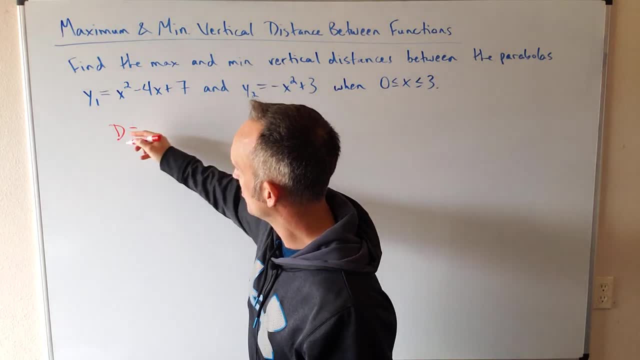 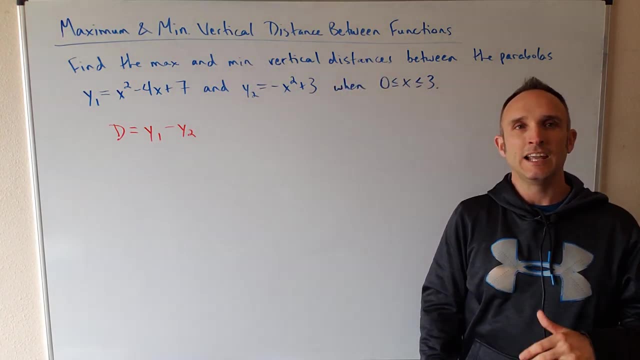 this guy is going to be higher than that guy. So what I'm going to do for my distance function, I'm going to take y sub one minus y sub two In. the problem with this is, with any optimization problem, the function you create. 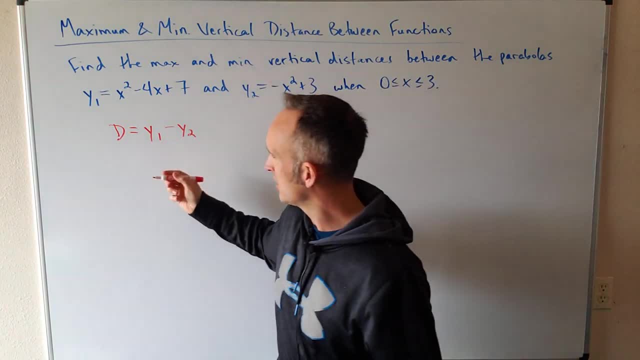 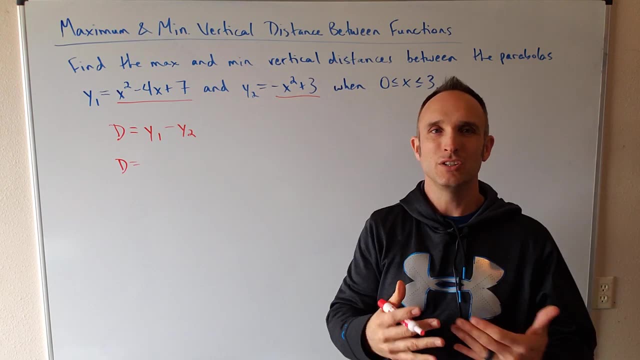 needs to be in terms of one variable. So, luckily for us, I can rewrite y sub one using x, and I can also rewrite y sub two using x. So I'm going to do that replacement. now, y sub one is x squared by x. Now, now. now, if we two of these are equal, we're each going to get one or the one. This is the problem with this problem. We say that one symbol is right here And we use x exactly in the moment when we're doing an operation. we say y by x, So there is an GORD of x, and we say y by x as a. 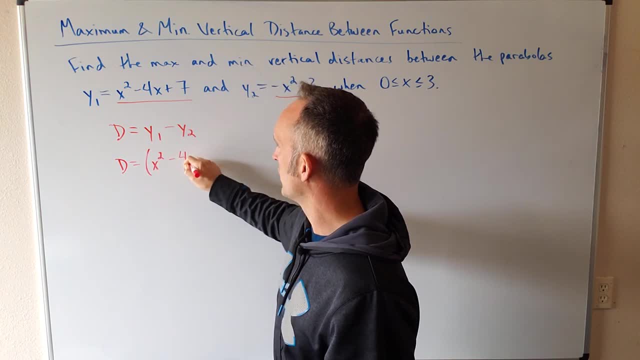 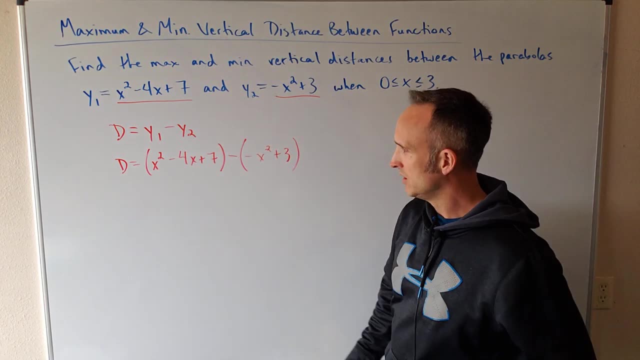 subscript in that term Now to get the function to visit and sold. So I'm going to do that. each function now: y sub 1 is x squared minus 4x plus 7 minus y sub 2 is negative x squared plus 3.. 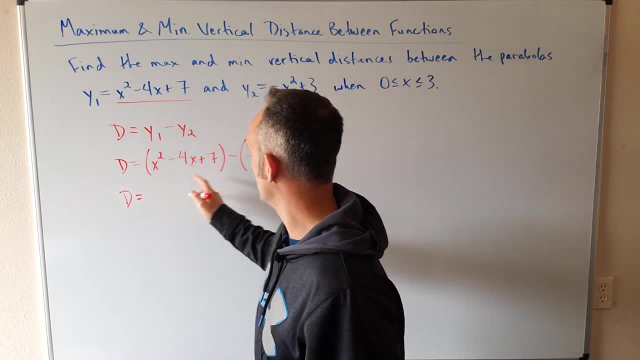 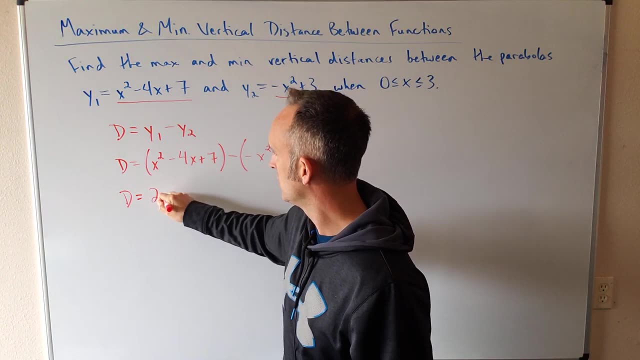 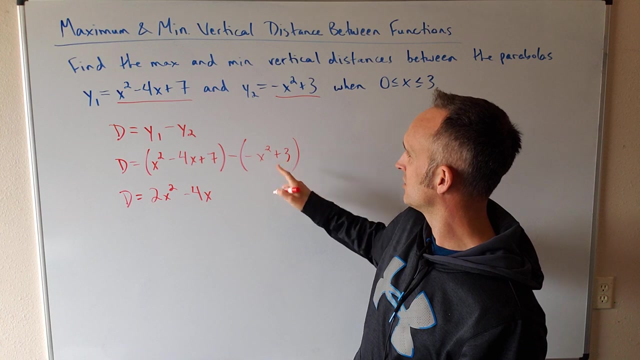 And so then I'll simplify this function a little bit by distributing my negative and combining like terms. So I've got x squared plus x squared, giving me 2x squared. Then I have negative 4x and I have 7 minus 3, which is positive 4, okay. 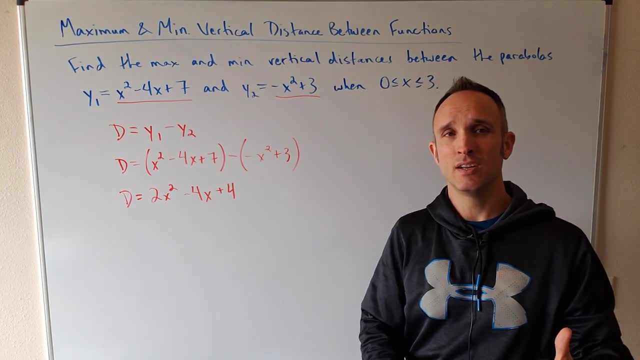 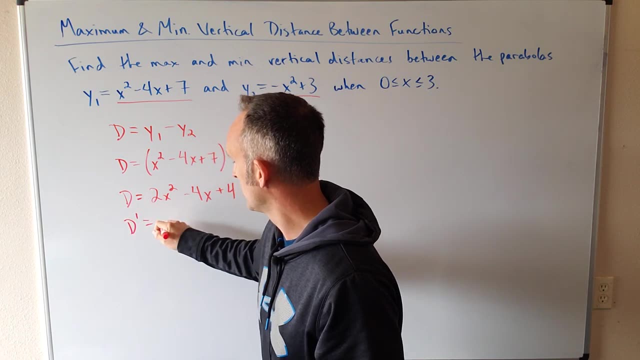 And so this is the function that we want to find the maximum and minimum of on the interval from 0 to 3.. In order to do that, I need to find its critical numbers, So I'll look for d prime, which will be 4x minus 4.. 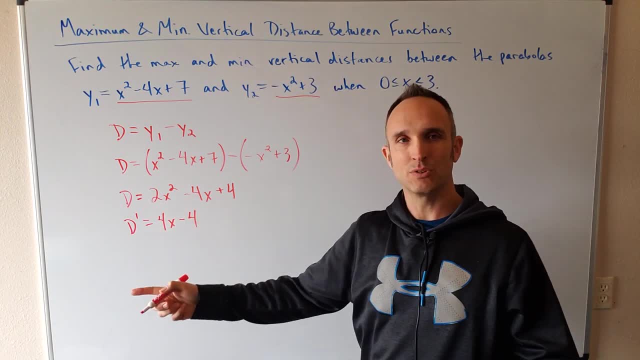 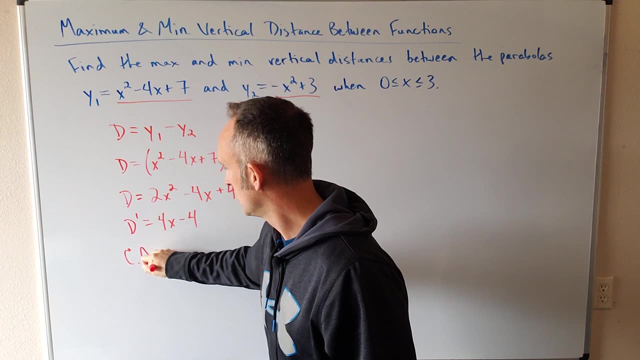 And so the critical number you can see is if this is 0. X would have to be 0.. X would have to be 1.. If you don't see that, solve that equation: 4x minus 4 equals 0.. 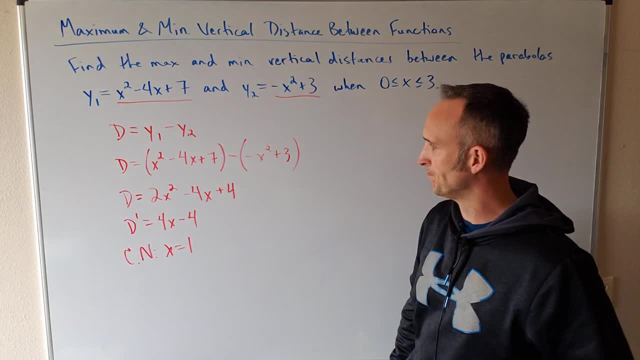 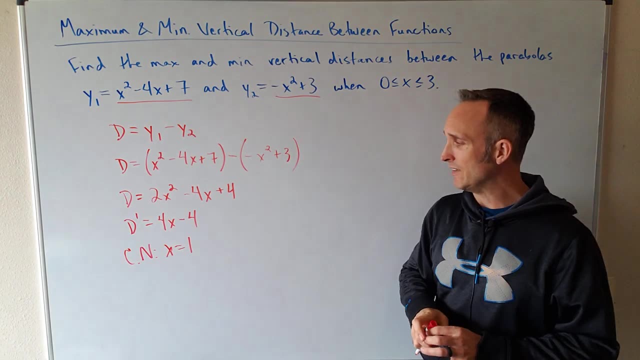 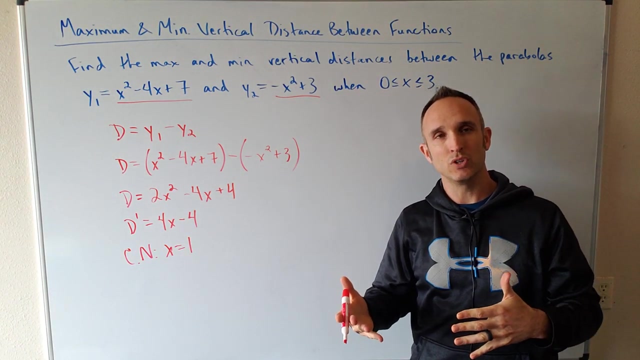 So the critical number is: x equals 1.. And good for us. this critical number lies in this closed interval, so that's useful. If it didn't, we would ignore it moving forward and we would only look at the end points of this interval by the extreme value theorem, which guarantees an absolute max and an absolute 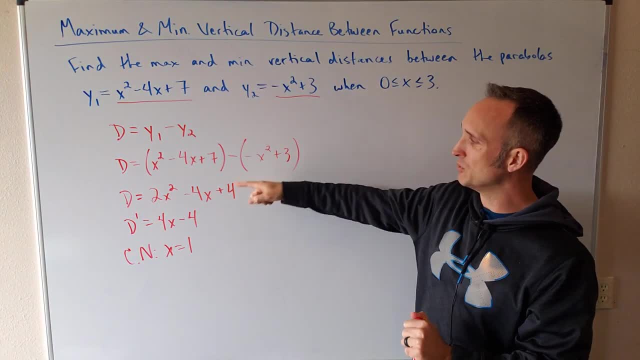 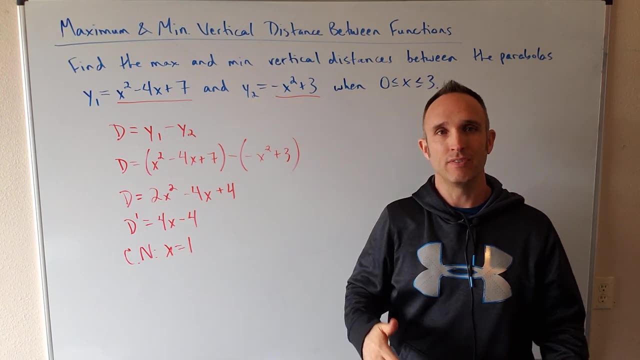 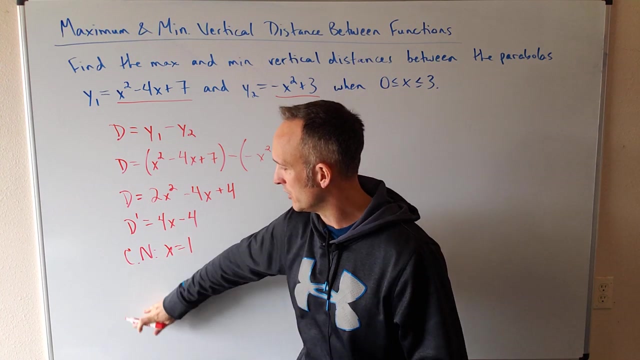 min on a closed interval For a continuous function at the end points or at critical numbers. If the critical numbers aren't in the interval, the max and min have to happen at the end points. But what we're going to do now is because of the extreme value theorem I don't have. 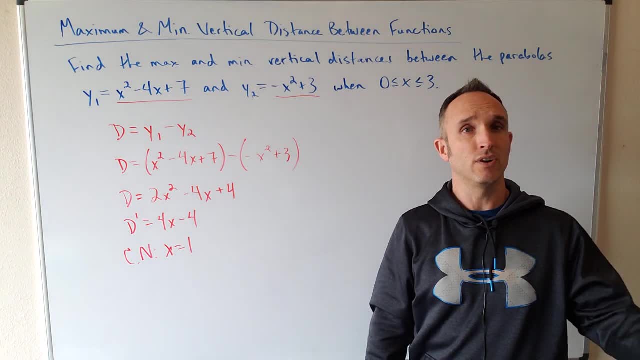 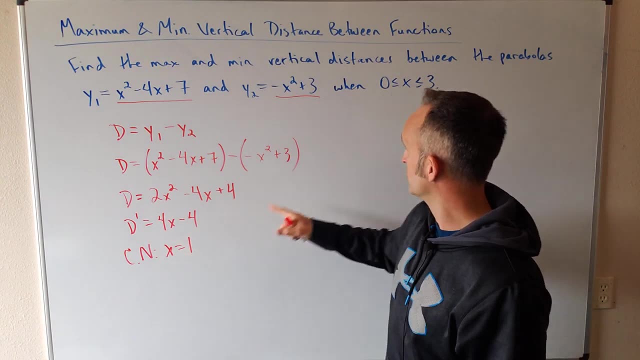 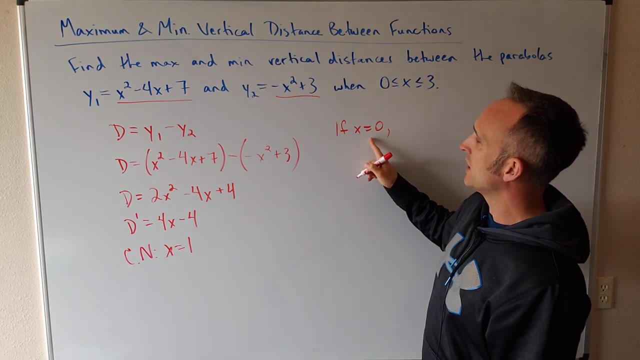 to look at my first derivative and find out where the function d is increasing and decreasing, because I know that I need to test. x equals 1,, x equals 0, and x equals 3.. So if x equals 0, we're trying to find the max and min vertical distance.